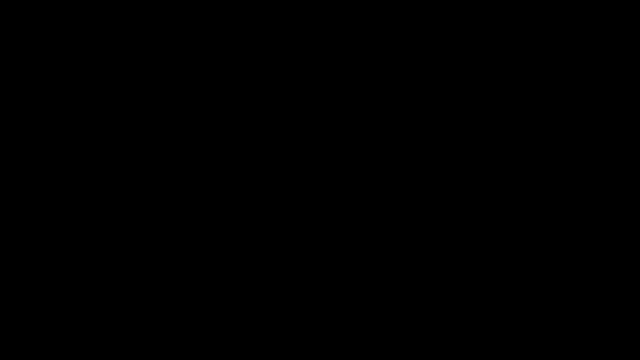 polar equation into a rectangular equation. So what is the difference between a polar equation and a rectangular equation? How do we distinguish the two? So here's an example of a polar equation. R is equal to 5 sine theta. A polar equation would have the variables R or theta A. 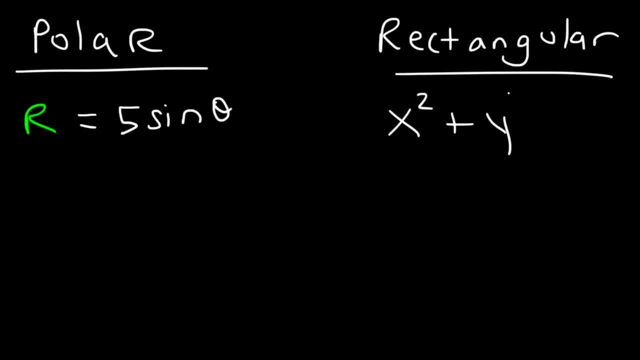 rectangular equation, on the other hand, consists of X and Y variables. So, for example, X squared plus Y squared is equal to 4. That's a rectangular equation. Another example is: let's say R is equal to a constant 7. That's a polar equation. Or X is equal to 3. That's a. 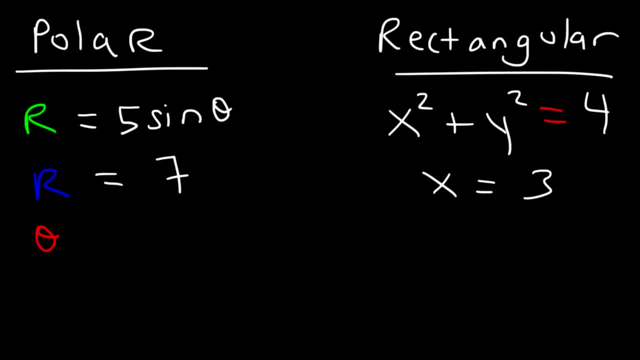 rectangular equation. Another one you might see is theta. Let's say it's equal to pi over 4, compared to X squared is equal to 4Y. So rectangular equations have the variables X and Y. Polar equations have the variables R and theta. 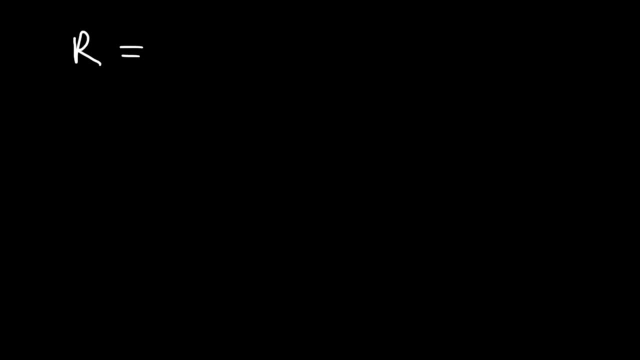 So let's work on an example. Let's say R is equal to 7. So convert this polar equation into a rectangular equation. So what do you think we need to do in this particular example? For each of these examples, pause the video and try it yourself, and then unpause it to see. 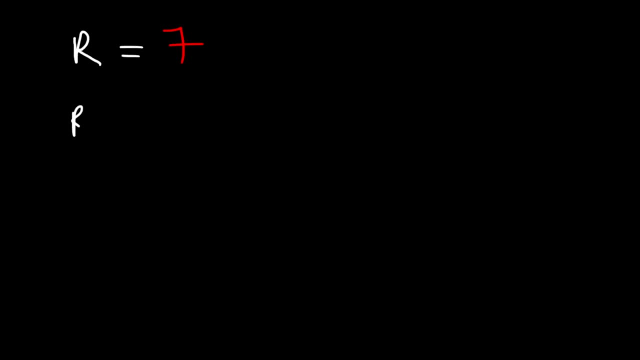 the solution. The best thing to do is take the square of both sides. R squared is equal to 7 squared, which is 49.. And, if you recall, X squared plus Y squared is equal to R squared. So therefore, X squared plus Y squared is equal to 49.. And that's all we need to do. 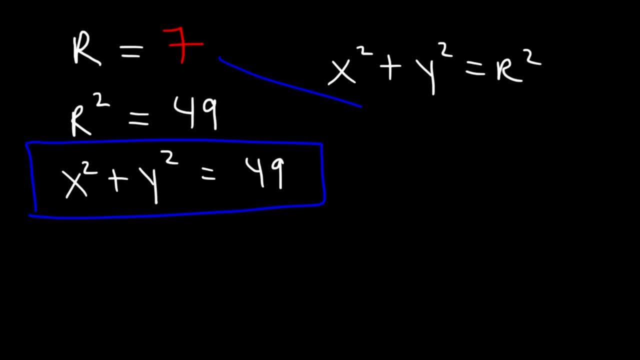 for this example. So that's how you can convert that particular polar equation into a rectangular equation. Here's another example. Let's say R is equal to 5. For the sake of practice, go ahead and try it. So we know that R squared has to. 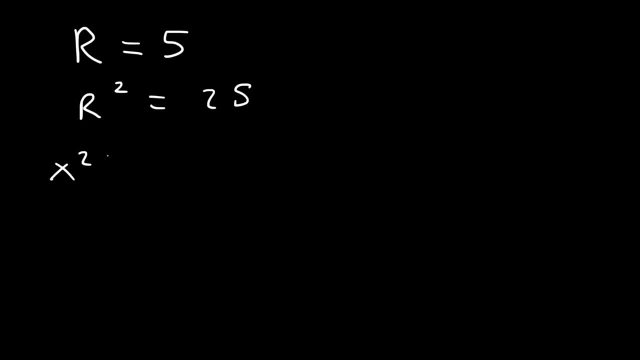 be 25, and X squared plus Y squared is equal to R squared, So that's equal to 25.. So anytime, R is equal to a constant number. that's what you need to do. Now. what if we have the angle theta? Let's say it's equal to pi. 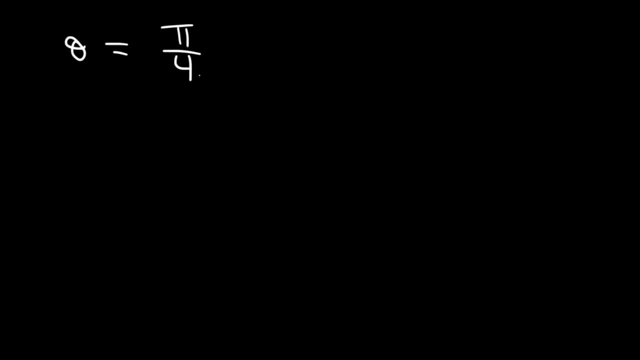 over 4.. Convert that equation into a rectangular equation. Now the first thing I would recommend doing is to take the tangent of both sides. So tangent theta is equal to tan pi over 4.. And, as you can see, the tangent theta is equal to tan pi over 4.. So the tangent theta is equal to tan pi over 4.. And as 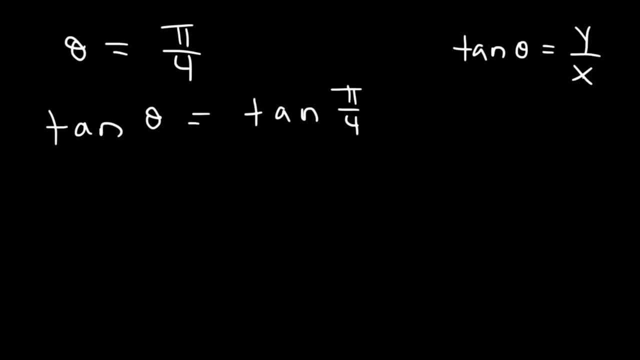 you recall, tan theta is Y divided by X. So that's one formula you want to keep in mind. So on the left side we have Y divided by X And tan pi over 4 is one. so all we need to do is multiply both sides by X. So therefore, in this example, Y is 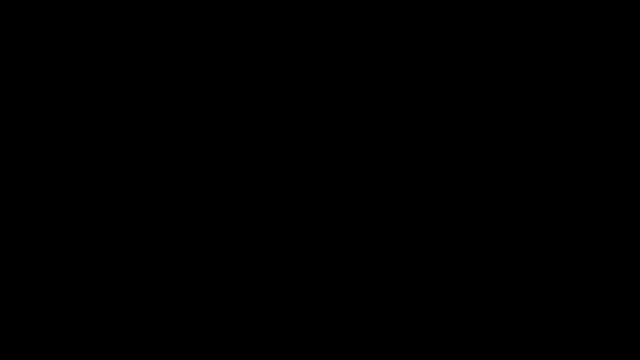 equal to X. Now how about this one? Let's say, if theta is equal to zero degrees, try that problem. so, just like before, we're going to take the tangent of both sides. so tangent theta is equal to tangent of zero degrees. and we know tan theta is Y divided by X. now what's tangent of zero? 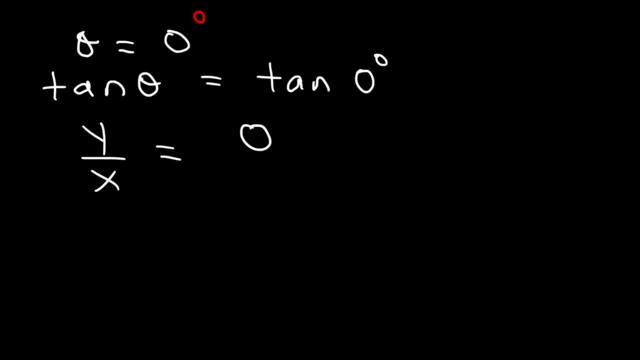 degrees tan, 0 is 0. now if we multiply both sides by X, these two will cancel, and so Y will equal 0. 0 divided by anything is 0, so 0 over 8 is 0, so it really doesn't matter what is the value of X. if Y over X is equal to 0, then Y 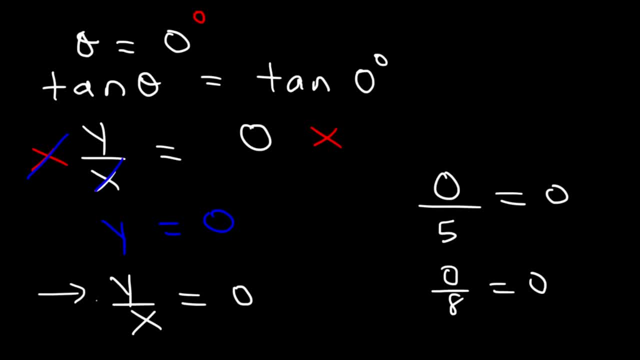 has to be 0. so this is the answer. now, what about this example? let's say: if theta is PI over 2, try that one. so we need to take the tangent of both sides. so tan theta is equal to tan PI over 2 and tan theta is: 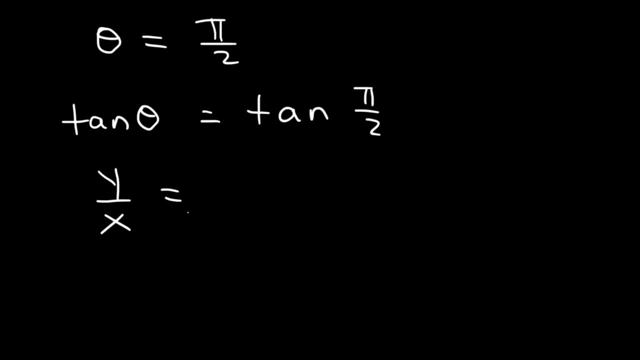 Y divided by X. now tangent PI over 2 is undefined. so if tangent PI over 2 is undefined, what do you do in this case? under what circumstances is a function undefined? a function is undefined if you have a zero on the bottom, if you have a. 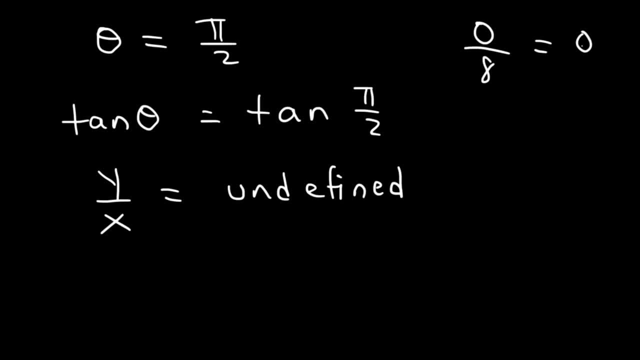 zero on top, the whole thing is zero. that's why in this example, Y was equal to 0. so if Y over X is equal to 0, Y has to be 0. but let's say, if you have 7 over 0, this is undefined. or 3 over 0, that's also. 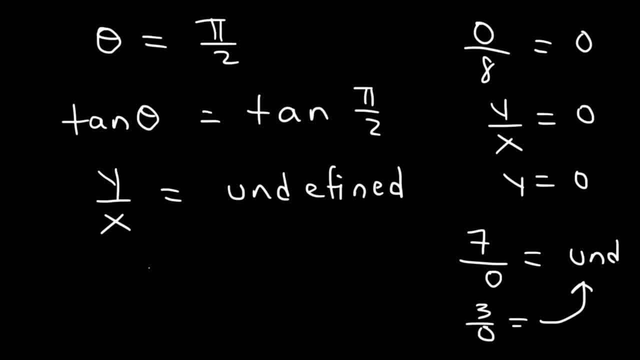 undefined. so, therefore, for something to be undefined, it's going to be some number n divided by 0, so we could say that X has to be 0. it doesn't really matter what Y is equal to, as long as X is 0, the whole thing will be undefined. 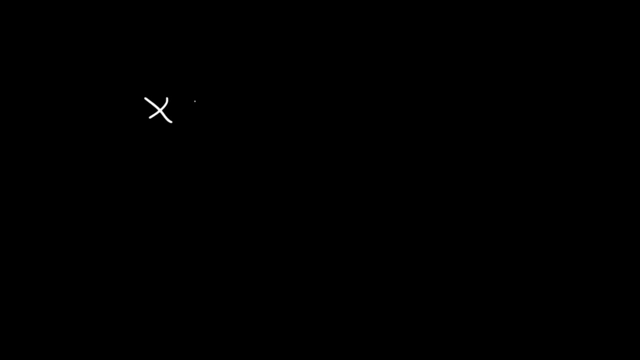 so therefore, the answer for that problem is X is equal to 0. let's say, if our sine theta is equal to 5 and also our cosine theta is equal to 4, convert each polar equation into a rectangular equation. so, if you recall, Y is equal to. 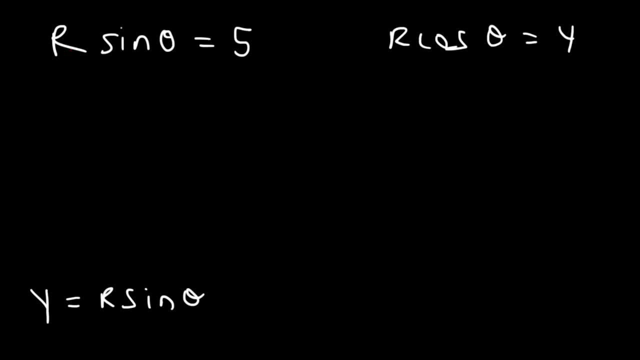 our sine theta. so therefore, we can replace our sine theta with Y, and this will give us the answer. so Y is equal to 5, and that's all you got to do now. for the other one, it turns out X is equal to our cosine theta, so we just got. 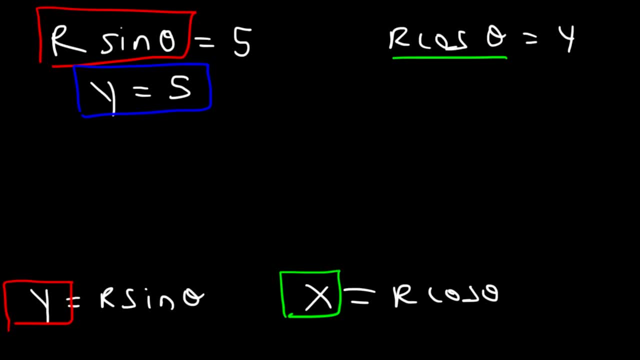 to replace our cosine theta with X. so the answer is: X is equal to 4, and so that's it for this problem. how about this example? let's say R is equal to 3 cosine theta. convert it into a rectangular equation. so cosecant is equal to what other? 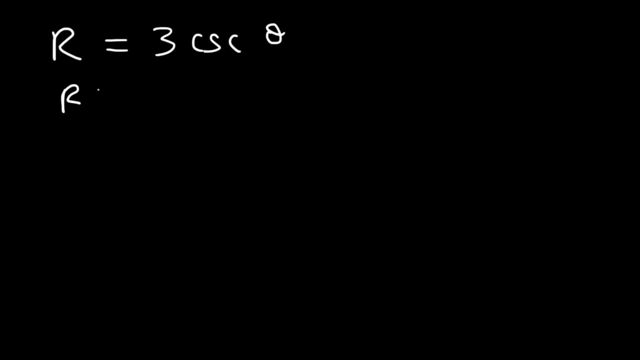 function, it turns out that cosecant is 1 divided by sine theta. so what we need to do is multiply both sides by sine theta. by doing so, we can get rid of the sine theta on the right side. so what we now have is R, sine theta is equal to 3 and 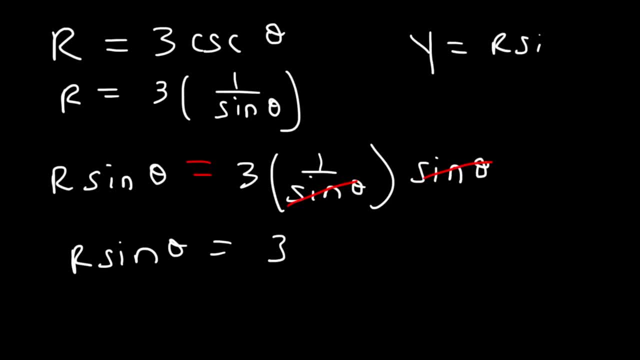 based on the last example, we know that Y is equal to R sine theta. so therefore Y is equal to 3, and so that's the answer for this problem. here's another similar question that you could practice on. try this one. let's say R is equal to 4 secant theta, so secant is 1 divided by cosine theta. 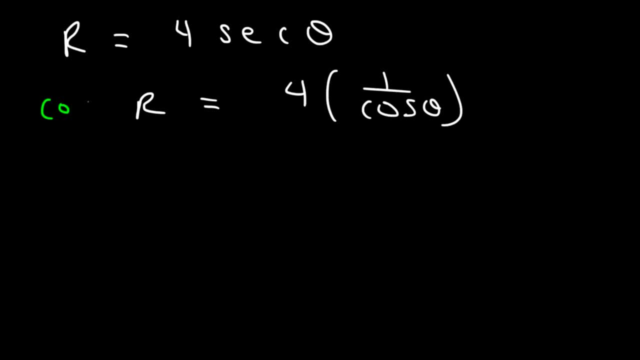 so now let's multiply both sides by cosine theta, so these two will cancel. R cosine theta is equal to 4. now we know that X is equal to R cosine theta, so therefore X is equal to 4, and so that's it. let's say if 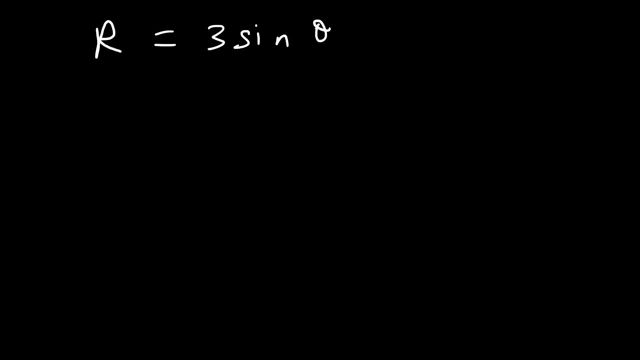 is equal to 3 sine theta. Try this one. What do you think we need to do in this problem? What I would recommend doing is multiplying both sides by r. Whatever you do to the left side, you must also do to the right side. So now what we have is r, squared is equal to 3r sine theta. 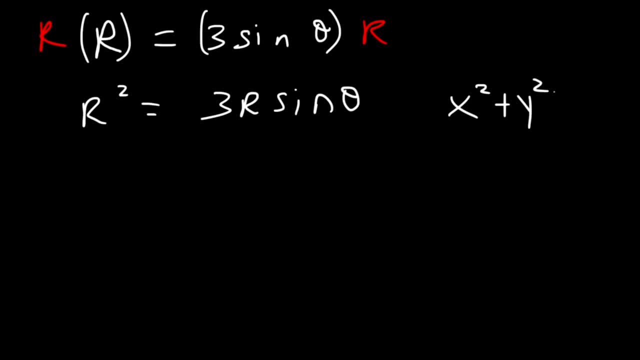 Now, if you recall, x squared plus y squared is equal to r squared, So we're going to replace r squared with x squared plus y squared. Also, we know that y is equal to r sine theta, So we're going to replace r sine theta with y. So 3r sine theta is equal to 3y. 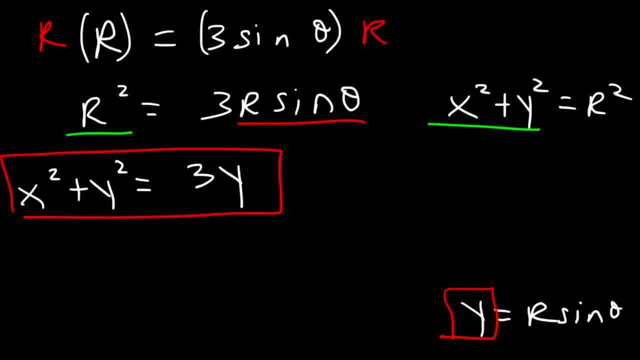 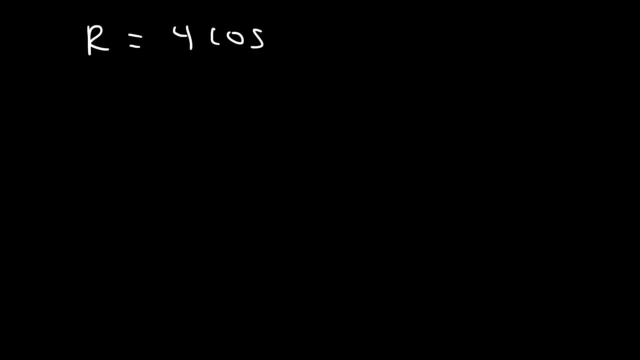 And this is the equation: x squared plus y squared is equal to 3y. So for the sake of practice, try this one. Let's say r is equal to 4 cosine theta. So, just like before, we're going to multiply both sides by r, So r squared is 4r cosine theta. 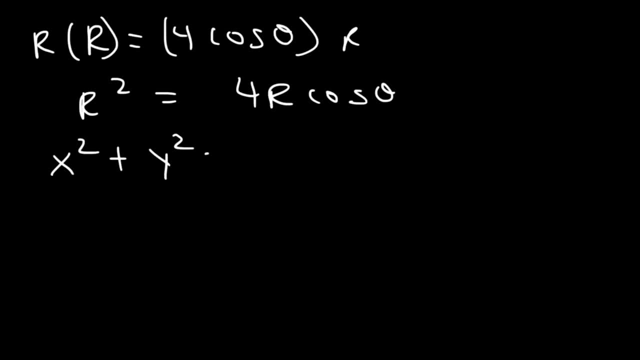 And r squared. we know it's x squared plus y squared And r cosine theta is x, So 4r cosine theta is 4x, And so this is the answer: x squared plus y squared is equal to 4x. 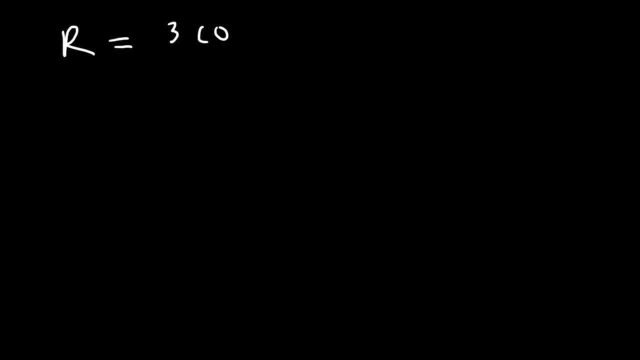 Try this one. Let's say, if r is 3,, 3 cosine theta plus 5 sine theta, Convert it into its rectangular form. So, just like we did before, we're going to multiply everything by r. So on the left side we're going to have r squared. 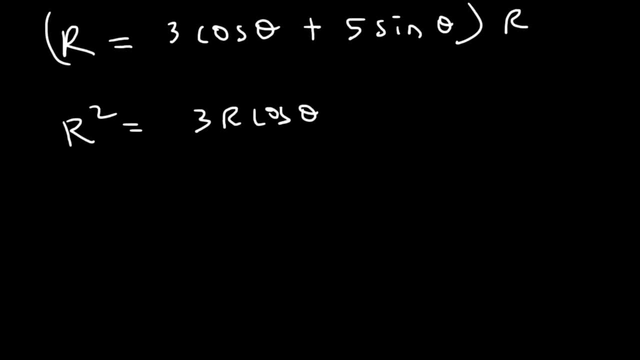 On the right side. we're going to have 3r cosine theta And then plus 5r sine theta. So we know that r squared is x squared plus y squared, And r cosine theta is x, So this is going to be 3x. 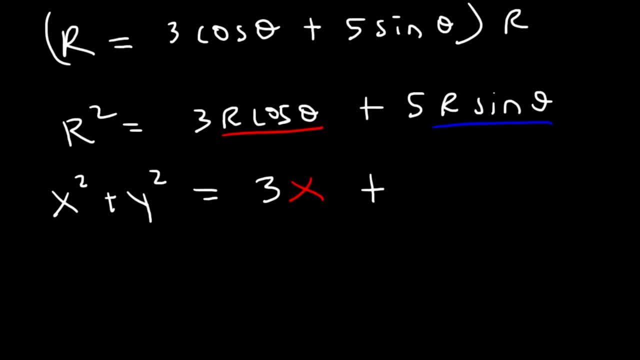 r sine theta, that's equal to y. So what we're going to have is 5y, And so that's the answer. x squared plus y squared is equal to 3x plus 5y. Let's try this one. Let's say if r is equal to 5y, 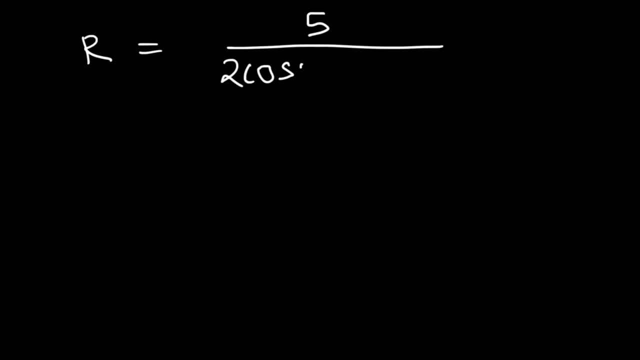 we're going to have 5 divided by 2 cosine theta plus 3 sine theta. What do you think we need to do for this problem? What I would recommend doing is multiplying both sides by the denominator of this fraction, That is, by 2 cosine theta plus 3 sine theta. 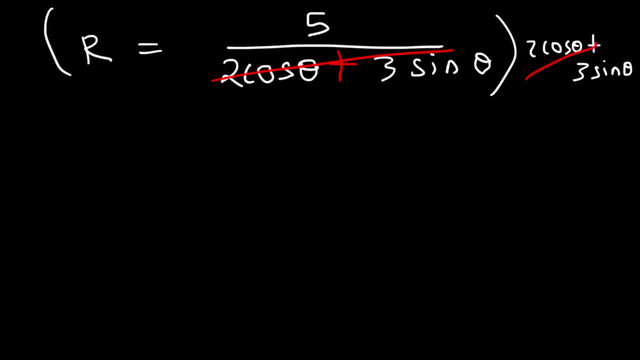 So on the right side that's equal to 5.. These two will cancel, But on the left side we're going to get r times 2 cosine theta plus 3 sine theta, And so all of that will be equal to 5.. Now what we need to do is distribute r. 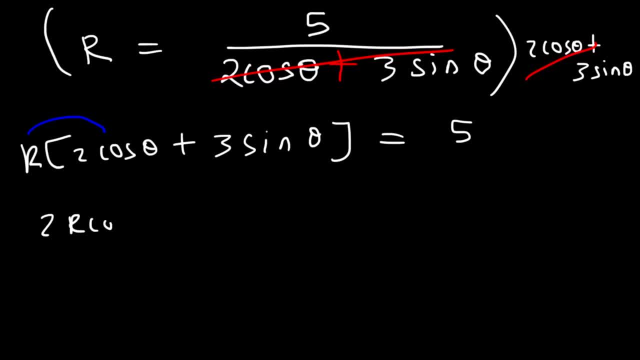 So what we're going to have is 2r cosine and then 3r sine, And that's equal to 5.. As you know, r cosine theta is x, So what we have is 2x And r sine theta is equal to y, So this is 3y. 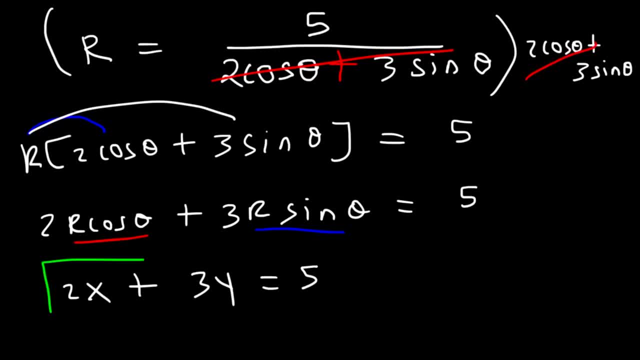 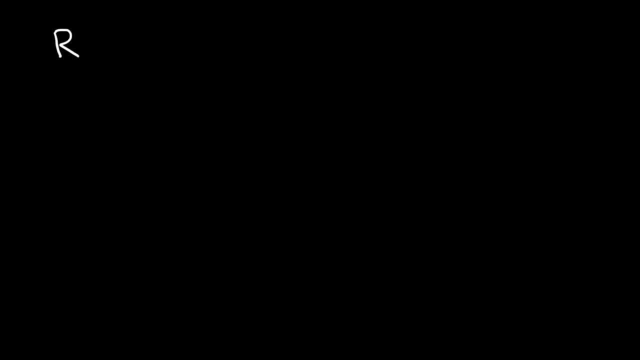 So we have a linear equation. in standard form, 2x plus 3y is equal to 5.. And that's the answer. Let's try this one. Let's say r squared sine 2 theta is equal to 8.. How can we change the equation? 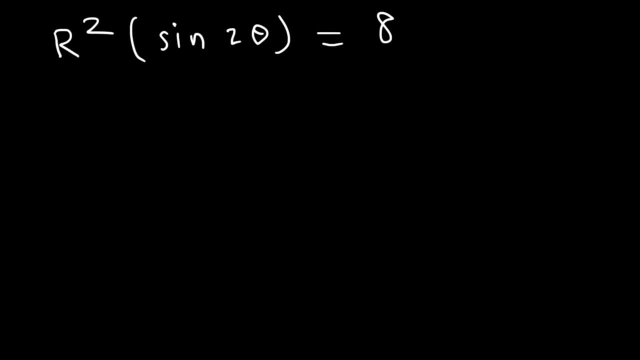 How can we change r and theta into x and y? for this particular example, The first thing you want to use is the double angle formula. Sine 2 theta is equal to 2 sine theta cosine theta. So this is going to be r squared times 2 sine theta, cosine theta. 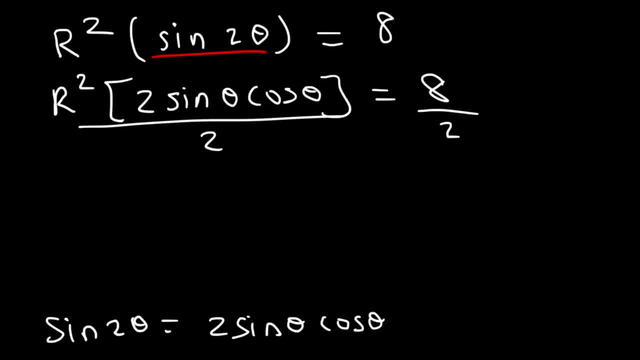 Next, let's divide both sides by 2.. So we can get rid of this number. So what we now have is r squared sine theta. cosine theta is equal to 8 divided by 2, which is 4.. r squared: we can rewrite that as r times r. 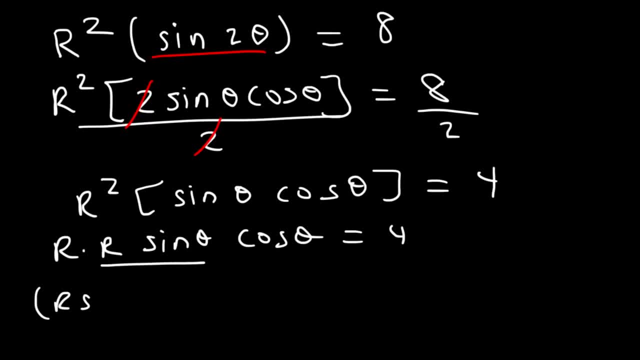 So I'm going to separate r sine theta and also r times r. So I'm going to separate r sine theta and also r times r. So I'm going to separate r sine theta and also r times r. So I'm going to separate r cosine theta. 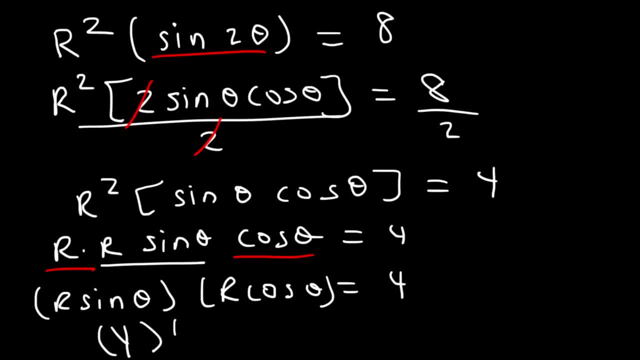 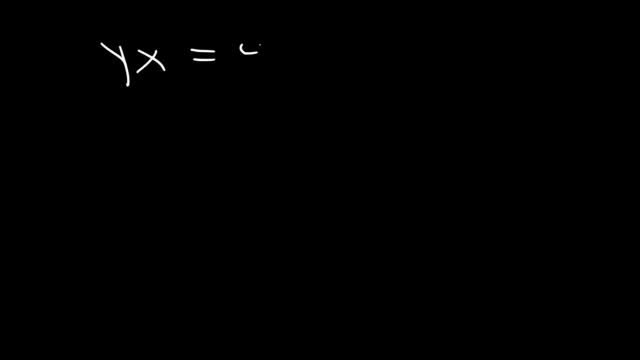 r sine theta is equal to y and r cosine theta is equal to x. So y times x is equal to 4.. If yx is equal to 4, then let's get y by itself. So therefore, y is equal to 4 divided by x. 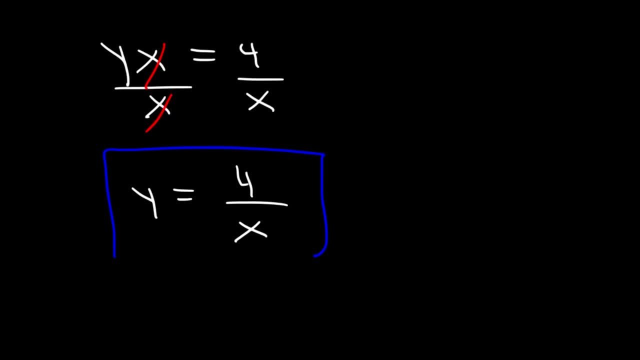 So we have a rational function And that's the answer. What if r is equal to 8 divided by cosine theta? What's the answer? In this example, what we need to do is multiply both sides by cosine, And we know that r cosine theta is x. 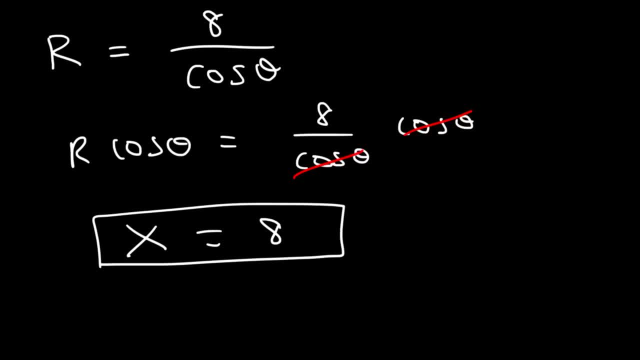 So x is equal to 8.. So that problem wasn't too difficult. Now what about this one? Let's say, if r is equal to 5 cosine theta divided by sine squared, What do you think we need to do for this problem? 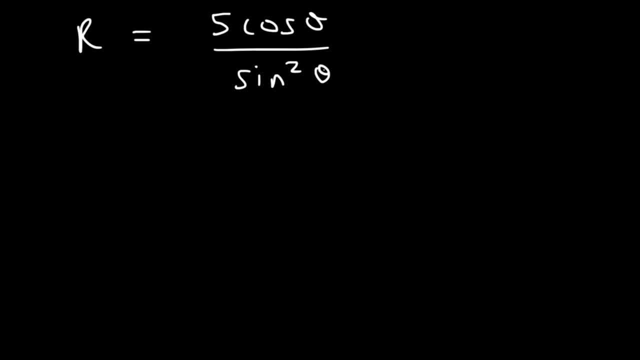 So feel free to pause the video and try it Now. what I would do is multiply both sides, not by sine squared but by sine theta, And you'll see why. So on the left, I have r sine theta, On the right, I have 5 cosine theta. 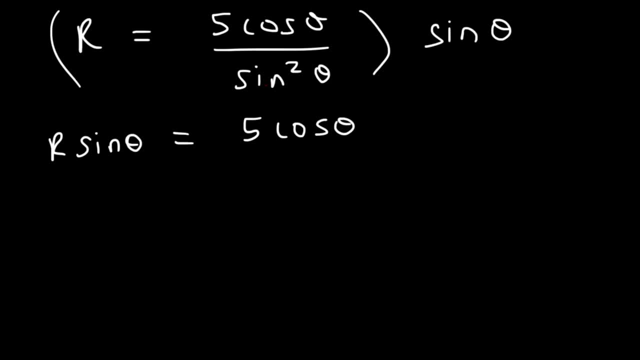 Now I had two sine thetas on the bottom, because it's sine squared And only one will cancel, which will leave one left over. So what we have is r sine theta is equal to 5 times cosine divided by sine. Now we know that tangent theta is y divided by x. 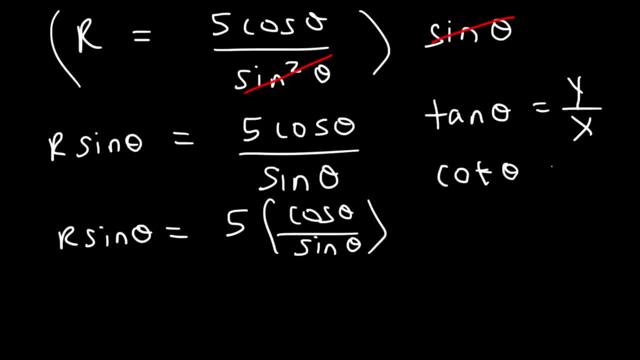 Which means that cotangent theta, which is 1 divided by tangent theta, is x over y. Now, cosine over sine Is cotangent theta And r sine theta. we know it's y. So y is equal to 5 cotangent theta. 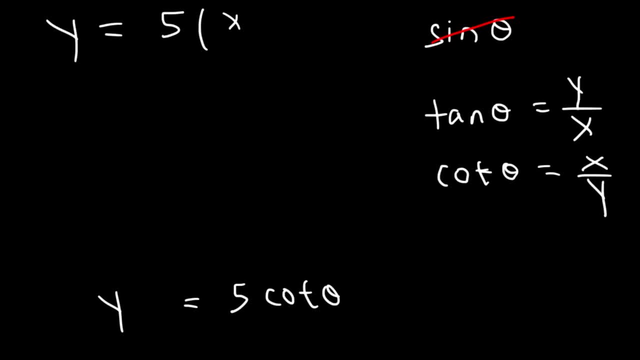 And cotangent theta is x divided by y. So now all we need to do is multiply both sides by y, And now we have the final answer: y squared is equal to 5x, And so that's the solution. Let's try one more example. 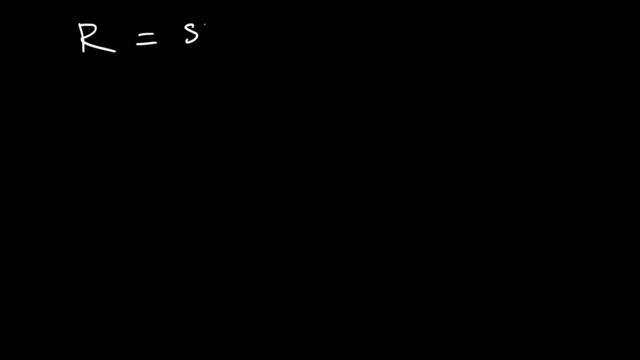 Let's say r is equal to sine theta, cosine squared theta. Let's convert that into its rectangular form. So what do you recommend that we should do? in the first step? The best thing to do, at least what I think to do- is to multiply both sides by r, cubed. 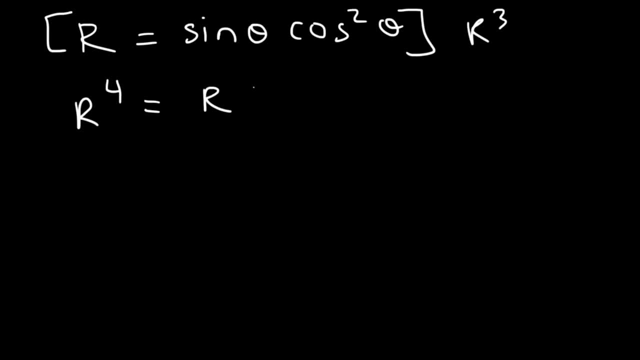 So, on the left, this is going to be r to the fourth. On the right, r cubed sine theta cosine squared. Now r to the fourth. I'm going to write it as r squared, squared r cubed. I'm going to expand it as r times r, times, r. 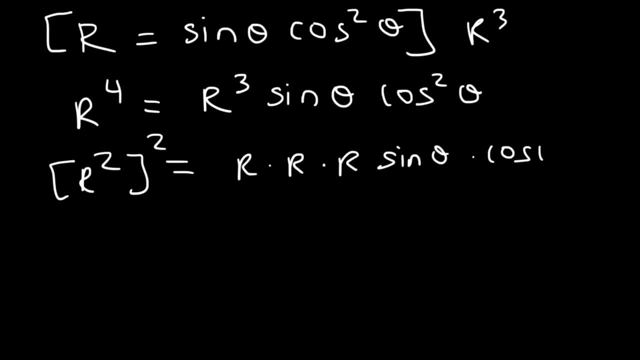 And cosine squared. I'm going to expand it and write it as cosine theta times cosine theta. Now I'm going to put these two together, So that's going to be r sine theta. And then let's put these two together, So that's r cosine theta. 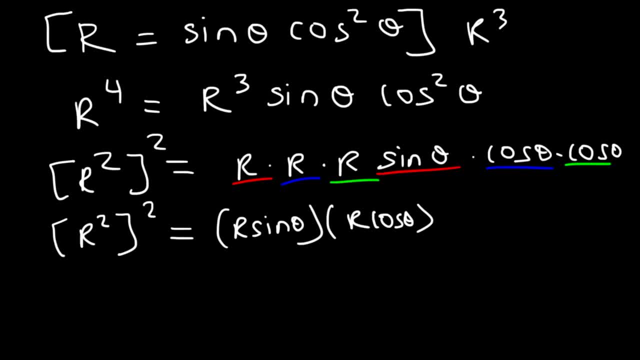 And let's do the same with the last two. That's r cosine as well. Now we know, r squared is x squared plus y squared, And all of that is raised to the second power. r sine theta is equal to y. r cosine theta is equal to x. 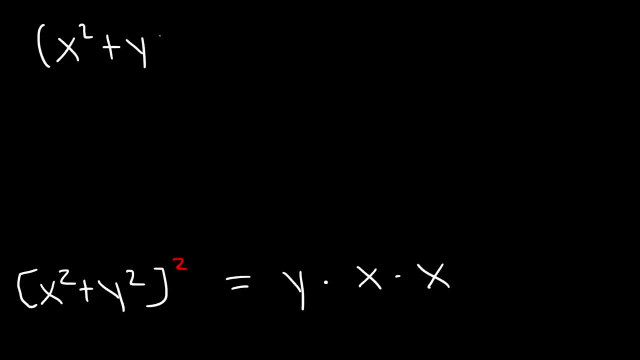 So what we now have is x squared plus y squared. squared is equal to y x squared. Now let's take the square root of both sides, So the square root will cancel with the square On the left. we're just going to have x squared plus y squared. 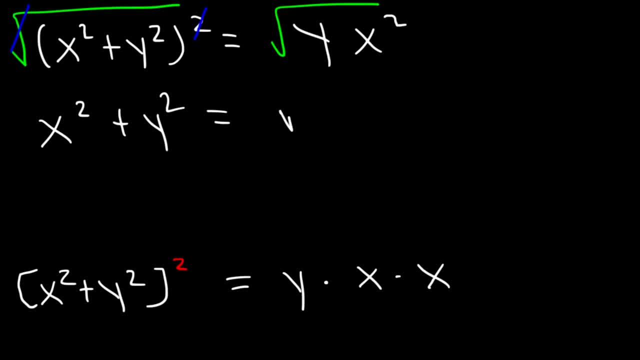 y squared On the right, we have the square root of y times the square root of x squared. if we expand it, The square root of x squared is x and we can't simplify root y. So this is it: x squared plus y squared is equal to x root y. That's the final answer. Thank you for watching.